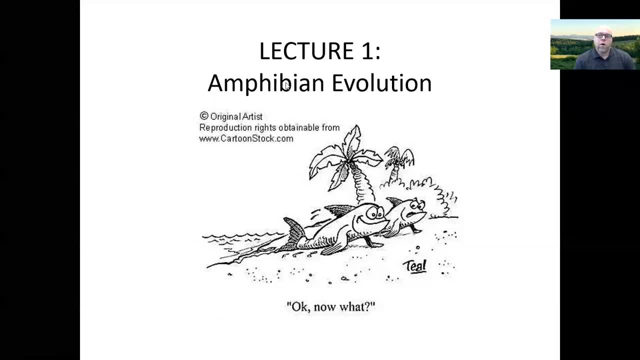 Welcome to the herpetology section of FNR 24150.. I'm Dr Williams. I'll be with you the rest of the semester teaching the herpetology section. I wanted to first just stop sharing my camera so that we can jump right into the lectures and you don't need to be watching me. I'd rather you watch. 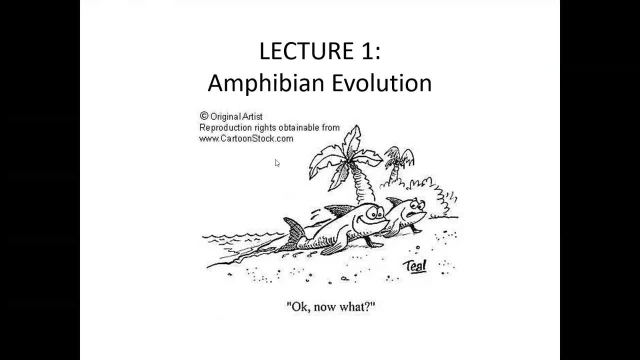 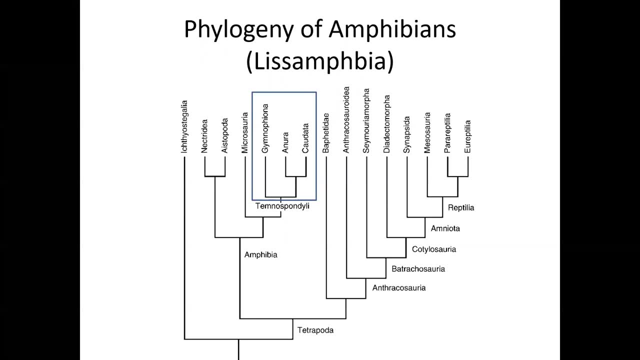 the slides at hand. So the very first thing we want to do is start thinking about amphibian evolution, So sort of get your bearings on where we are in terms of our extant amphibians. If you look at this blue box that I have listed around the temnospondyly, you'll see Gymnophiona. 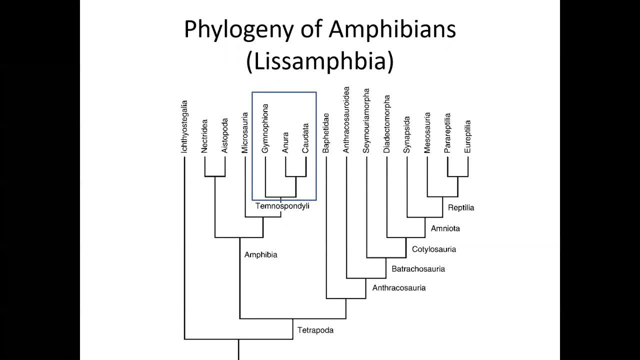 Anura and Caudata. Those are our extant amphibians within the group called Lysa amphibia. But one of the things I really want to show you in this cladogram is a focus here on this split of Tetrapoda. What I want to point out is just: 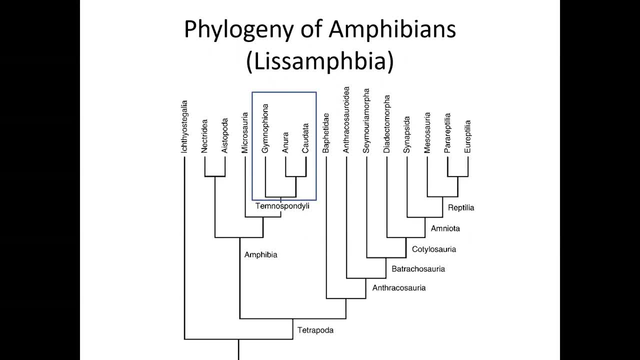 how disparate, just how distant, distantly related the amphibians are from our reptiles. So you can see the branch of the tetrapods leading to amphibia, the temnospondyly, and again our Lysa amphibia, Whereas the other branch of the tetrapods go to Anthracosauria, Patrachiosauria, Caudaliosauria. 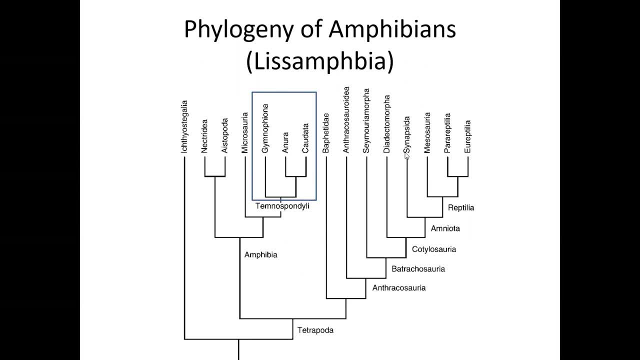 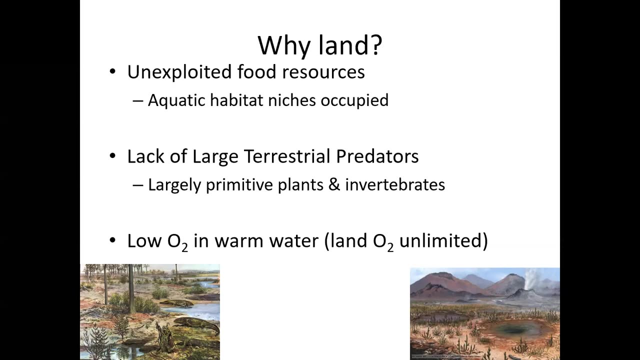 and Neota, which lives in Synapsus, which is our modern day mammals, and then our reptiles, And so you can see again just how distant these particular amphibians are from our reptiles. The question you might ask yourself is: why land in the first place? So one of the things that Dr Christy probably left off with was the Sarcoptaginia and Lobe-thin Fishes. 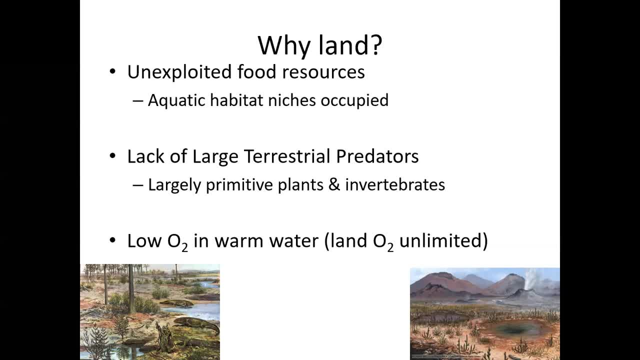 And that's really where our story begins, here with herpetology, And we try to figure out why we had these vertebrates that inhabited the waters. why did they transition on into land? Well, there's lots of different hypotheses and I'm just going to highlight three. 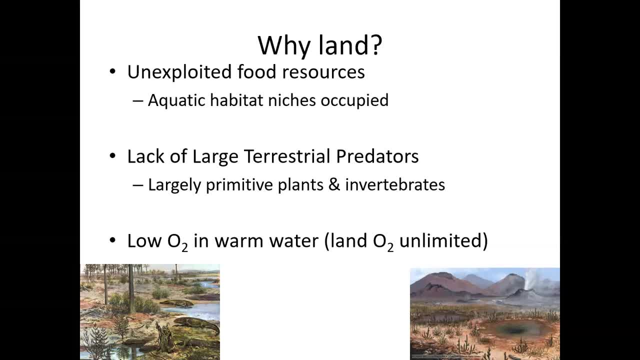 So the very first one is unexploited food resources. So, if you think about it, most of the aquatic habitat niches were occupied by large predatory fishes and other chondrichthys sharks. So when you think about the land, there was a complete lack of large terrestrial predators. The land was primarily made up of primitive plants and invertebrates. 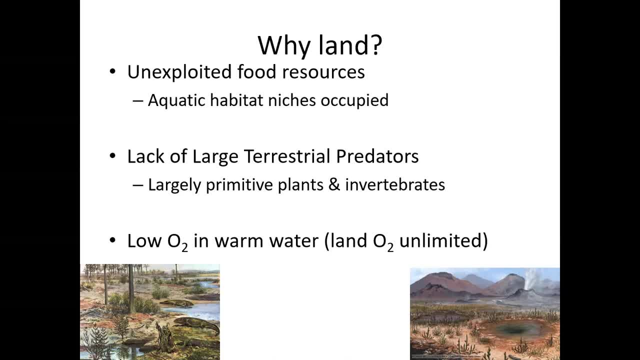 So there was really very limited competition on land Relative to the fully occupied niches found in aquatic settings. Another hypothesis regarding the emergence of land for these really early amphibians and tetrapods evolved from air breathing fishes in these swampy habitats with really low oxygen content, which favors emergence on land, where obviously on land oxygen is nearly unlimited. 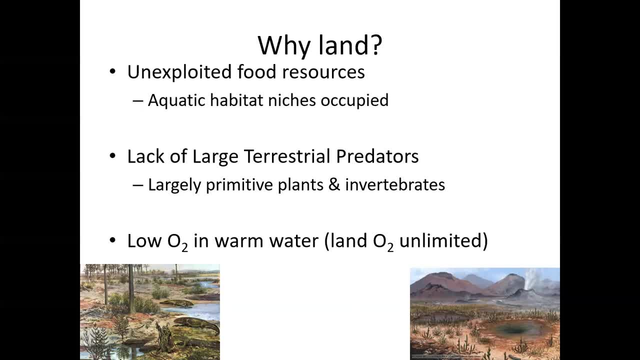 And this corresponds to when we see some of these large radiations that we're going to talk about later in lecture. When you think about the Permian, we started having this really droughty conditions, which made it suitable for some of these animals that could make small traverses across different evaporating pools of water, able to excel in that particular climate. 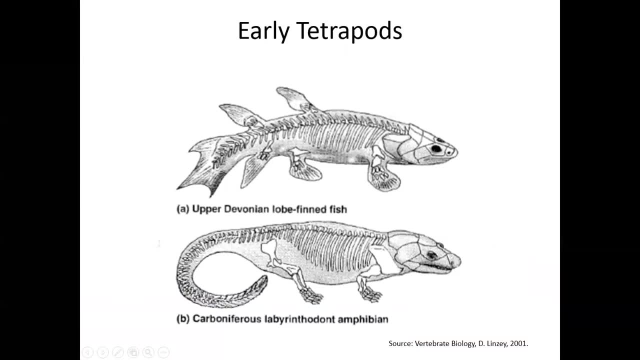 So let's take a look at some of these really early amphibians, or tetrapods, relative to these upper Devonian lobefin fishes. Remember, these are Sarcopterygian lobefin fishes. One of the very first things you're going to note is that they, in these lobefin fishes, they have these median fins, whereas on our Carboniferous labyrinthimodont amphibian, we lack those median fins. 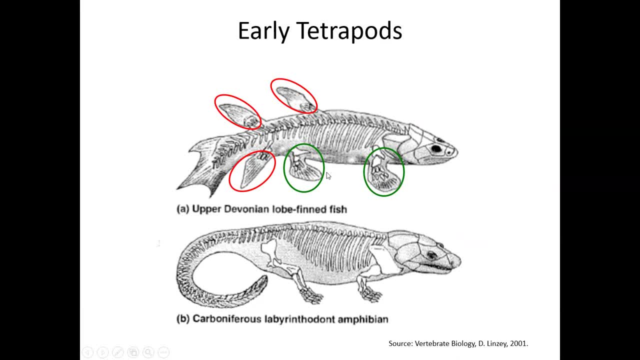 You also see these pelvic and pectoral fins slowly transition into paired paddles, like going from paired paddles into limbs. You're also going to note a a really large increase in the size of the ribs And again, this is to support. 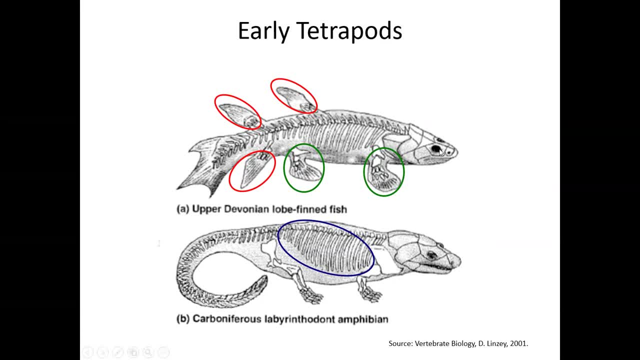 the internal organs because, if you think about it, if you're in the water, your organs and your body weight is largely supported by the water itself. Once you move on into land, you need to increase your skeletal system to help support those internal organs. 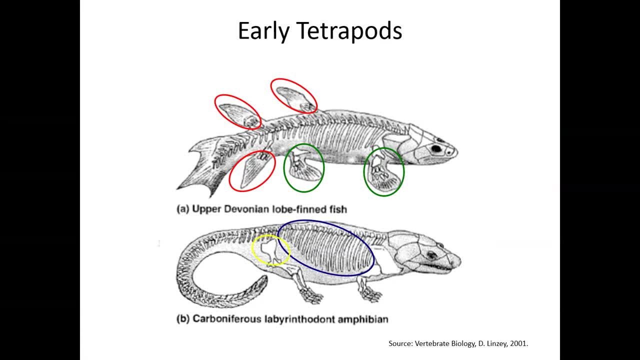 And the last thing: if you look at the pelvic and pectoral girdles in our labyrinthimodont amphibian, much, much larger pelvic and pectoral girdles, again to increase the area for muscles, because those muscles need to be stronger to support the animal's weight once they move on into land. 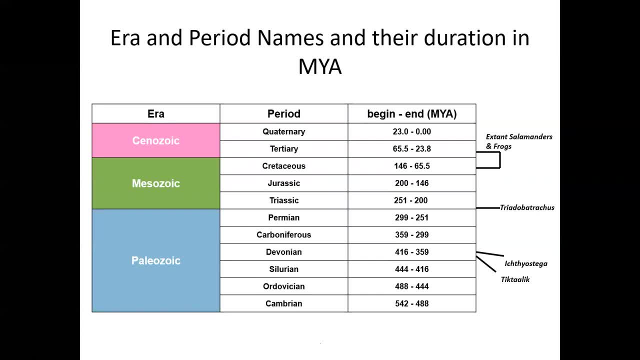 This is the table that you're going to want to think about and refer back to many times throughout the semester, because it does a really great job of outlining the areas, the periods and where some of these really important fossils, like our Tictolic or Ichthyostega, happen to show up throughout. 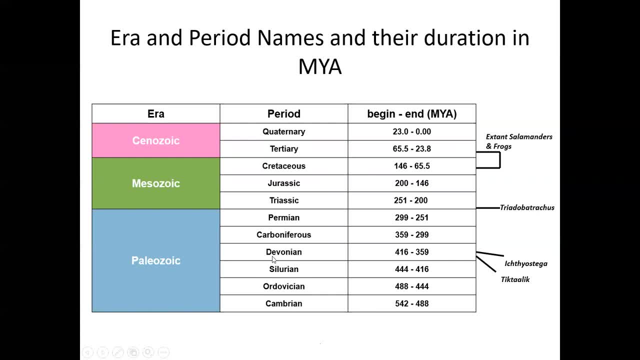 these epochs and eras. So again, our story really begins in the Paleozoic era and the Devonian period, And again I have listed here some of the really major events that I want you to at least be thinking about as we start talking about some of these really important fossils throughout the lecture today. Those are Tictolic Ichthyostega Tridobitrachis, and when our extant frogs and salamanders began to emerge onto the scene. 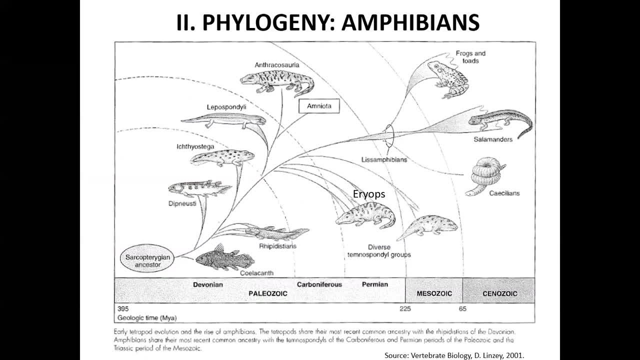 So this is a picture of our. This is a different pictogram, really highlighting when a lot of this major evolutionary transitions happened over the last 350 years. Again, Dr Christie talked to you about the Sarcopygenean lobedent fishes, which are the ancestors to all tetrapods. 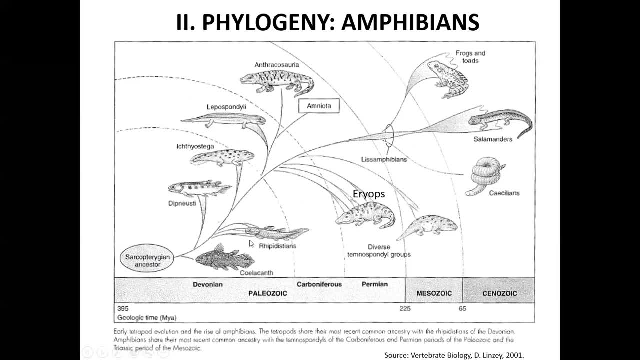 So we're going to start going through some of these phylogenetic relationships. Now, remember, these phylogenetic relationships, particularly with amphibians, are a little bit spotty because some of these amphibian skeletons are really far from each other. 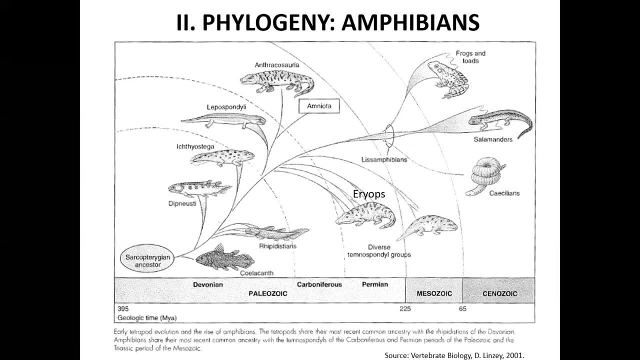 are really small, and so we have large gaps, And so this is our best representation of how we think we move from Sarcoptagian lobe-thin fishes into our extant amphibians and reptiles of today. So again, our story is going to begin in the Paleozoic era, in the period in the Devonian. 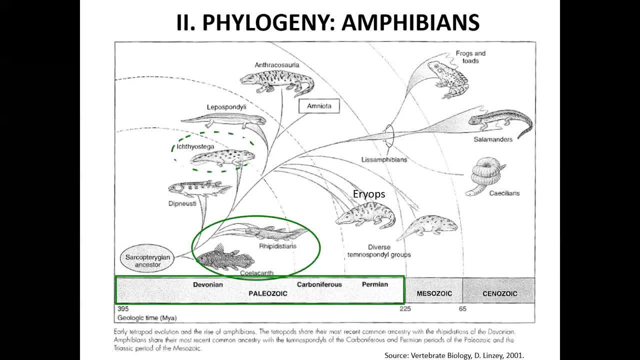 And some of our very earliest fossils of these early tetrapods amphibians. one of these is the ichthyostegans, The earliest known amphibians. they had short, stubby legs, five toes and a tail fin. They had scales on their bellies and tails- Most early amphibians. 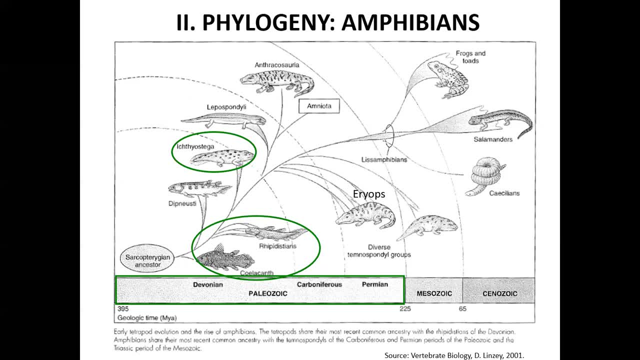 were much larger than species that exist today. In fact, some of these were up to 15 feet long and fed on large insects because, remember, during this time there were no predatory mammals on land. These were the dominant land animals for at least 75 million years. 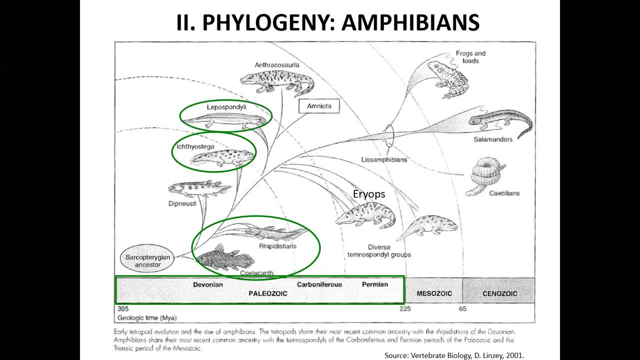 Now, if we move on into the Lespedondyli as well as the Temnospondyli, we're going to start moving into the Carboniferous period. So the Lespedondyli are a group of very small yet very diverse early 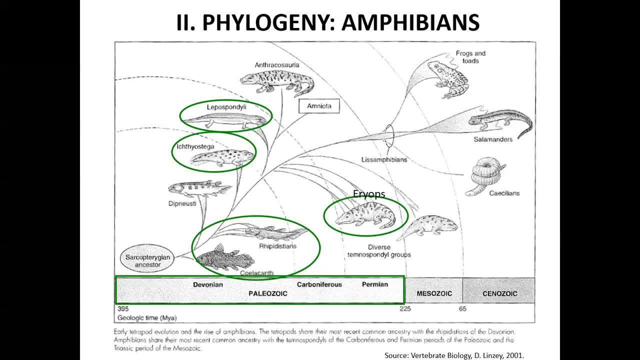 amphibians. They include animals that are newt-like, eel-like or even snake-like in lizard-like forms, along with a bunch of species that really don't fit any categories. Now, obviously, as you can see from this picture here, this is an evolutionary dead end. None of the animals from this particular lineage are extant. 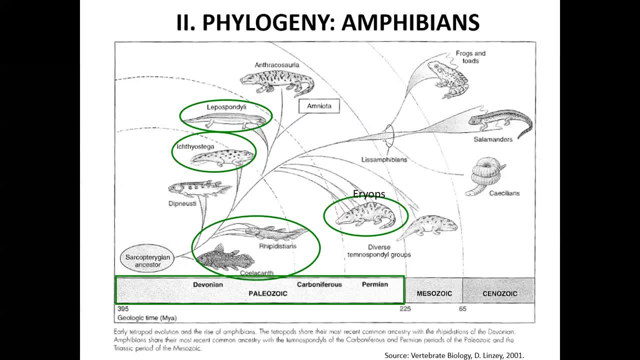 today One of the most well-known fossils that we have. it's called a Diplocollis and I'll show you this fossil here just a little bit. but it belongs to the Lespedondyli group that again had a lot of. 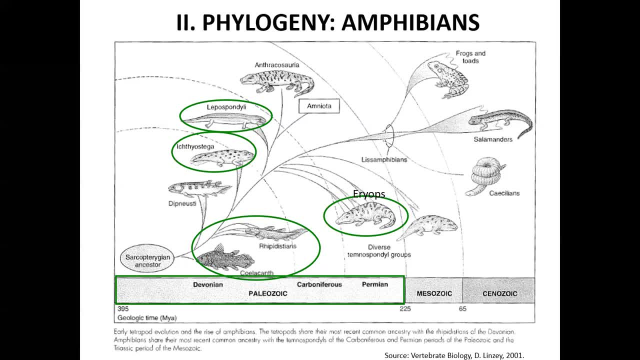 diversification in the Carboniferous period, but didn't really make it into the Permian. If we think about the really diverse Temnospondyli, another extinct group of labyrinthinodont amphibians, Some of these were carnivorous, were completely aquatic, while others walked on land as adults. And the size. 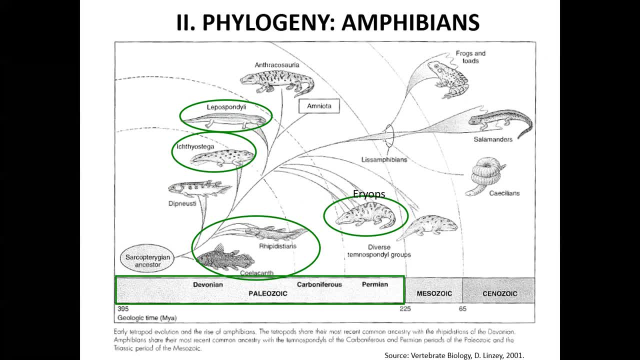 variation of the Temnospondyli is really really large, from something that's less than six inches in length up to 31 feet in length. The front feet had four toes, the rear feet had five toes, And these Carboniferous lived into the late Mesozoic era And some of the 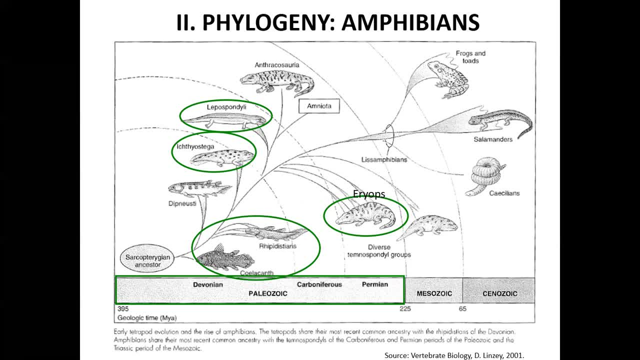 Temnospondyli included things like our Eriops, which we're going to show you a fossil here in just a little bit as well. Now, one of the things that I want to point out is here in the Carboniferous, we also have these lineages of Anthracosauria, as well as Amniota, And it's this Amniota branch. 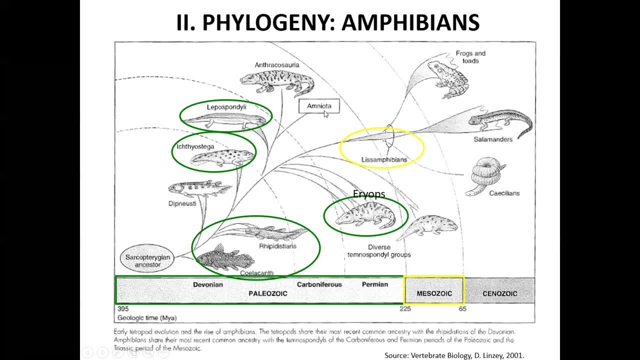 that we're going to talk about in a couple of days, when we start talking about reptilian evolution, which started in the mid to late Permian. But remember, in the Permian we started to see really droughty conditions, which is when a lot of our reptile and early 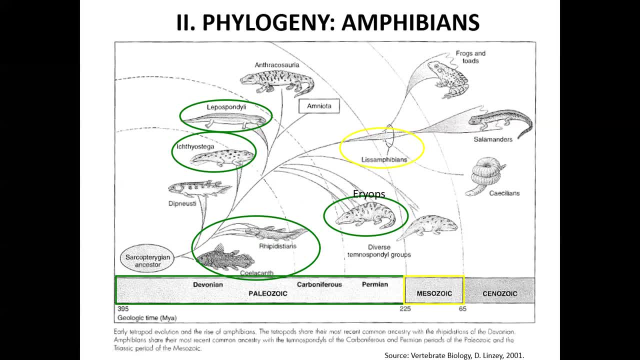 reptile species began to emerge and evolve Because, in general, they tend to be adapted to more arid climates than our amphibians that are really tied to moist environments, And it really wasn't until the latter part of the Permian that we get this little mini radiation. 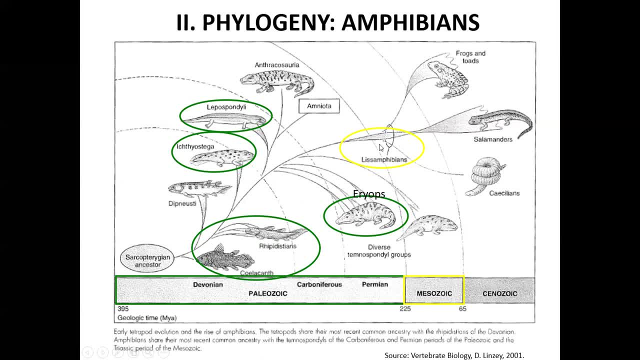 of amphibians, And this is actually where our Lyssa amphibians emerged, toward the end of the Permian and the early portions of the Mesozoic, And it wasn't until the Cenozoic when we started to get rapid expansion in the current day amphibians that we have today represented. 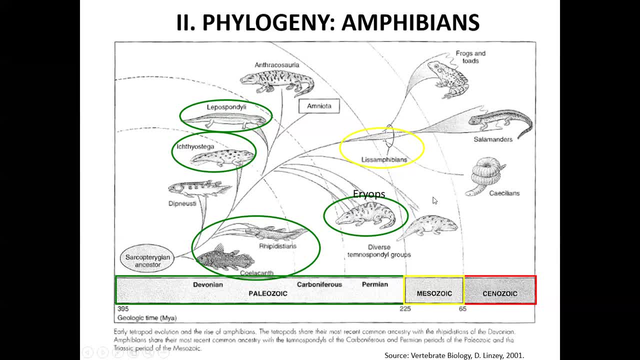 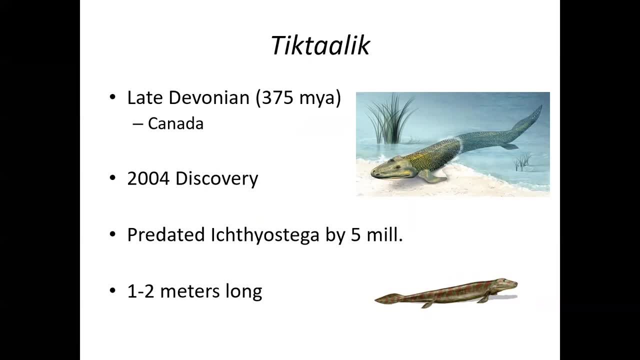 by our Nurans, our frogs and toads, our salamanders and our caecilians. So let's jump in and start talking about some of those really important fossils- And I'm not going to show you all the fossils, but the ones I do show you are important. 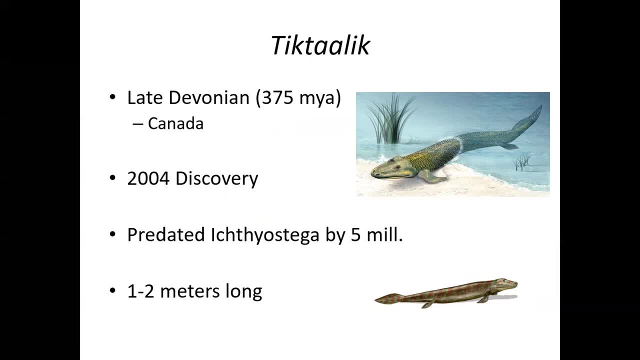 and will likely come up in class discussions, quizzes and perhaps your final exam. So it is important to know the characteristics of these fossils. So the very first early tetrapod fossil is called Tiktaalik. It was discovered in Canada in 2004 and it actually predates the previous fossil by about five million years, which was 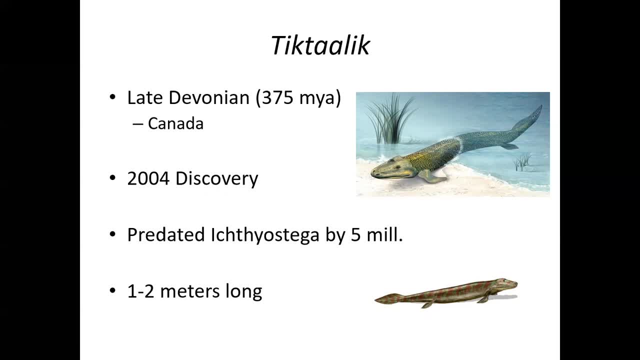 the Ictalipod. The Ictalipod was the first fossil that was discovered in Canada in 2004 and it actually predates the previous fossil by about five million years, which was the Ictalipod. So this particular fossil, the Tiktaalik, was one to two meters long. 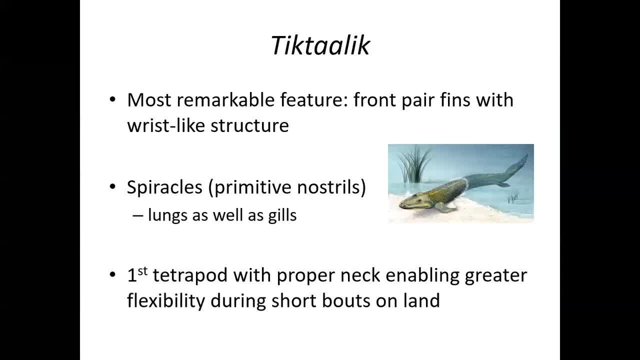 and it had some really interesting features. The most remarkable was paired fins with wrist-like structures, which again allowed it to perhaps make short trips onto land as we start moving from that Devonian into the Permian, when again we start having these drying conditions. 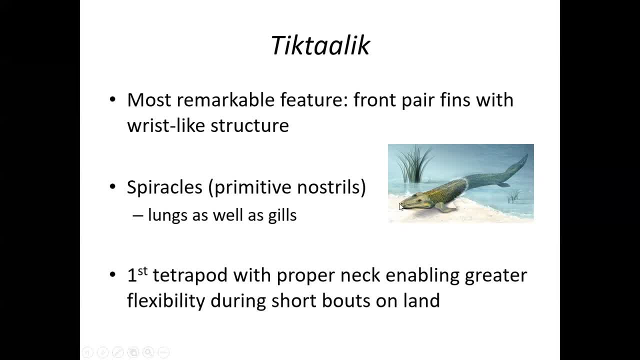 They also have primal, primitive nostrils, which are termed sphericals. They also have lungs as well. This was the very first tetrapod that had the proper neck, which enabled it to have greater flexibility again during these really short bouts of time that it might spend on land. 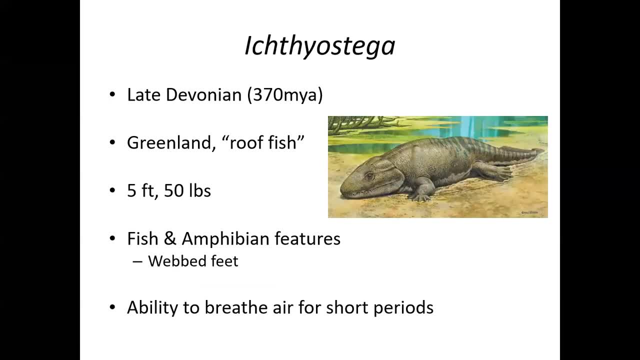 moving from one evaporating body of water to the next. Icthyostega was some five million years later in terms of fossil dating. in the late Devonian It's called the roof fish. It was anywhere from five pounds or five feet long, a weight up to 50 pounds. It has both these fin. 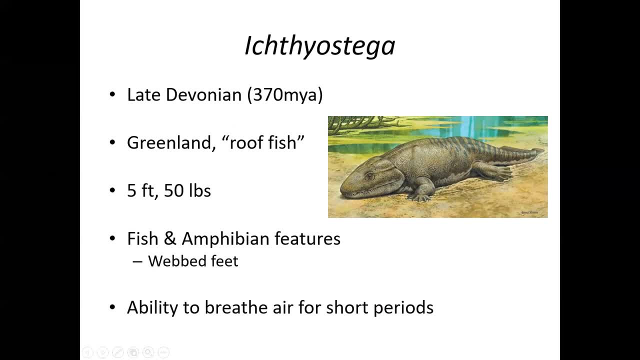 fish and amphibian-like characteristics. So the amphibian features had these webbed feet, the ability to breathe air for short periods of time, and this early tetrapod was also thought to have been able to haul itself on the shore for these really short periods of time. 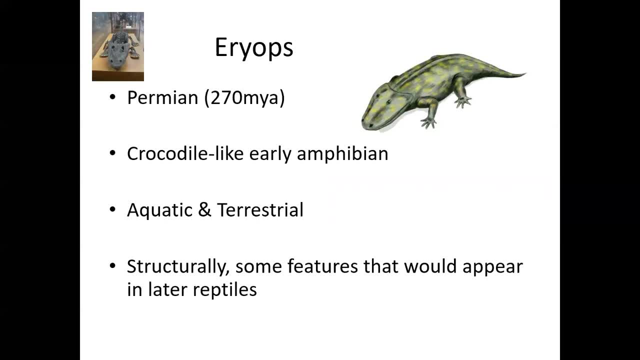 Here we have Eriops. So now we've launched ahead about 100 million years of evolutionary geological time. So now we're in the Permian 270 million years ago And when you look at the skeleton of Eriops it actually has a lot of crocodile or crocodilian-like. 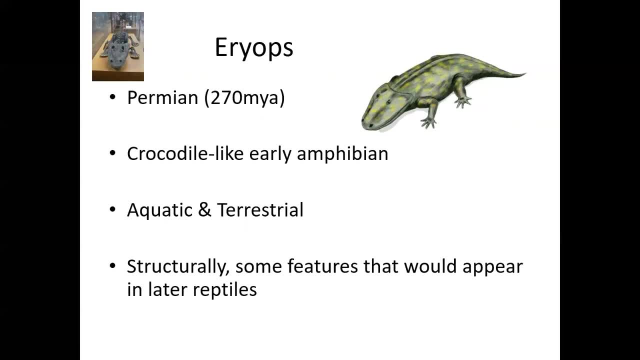 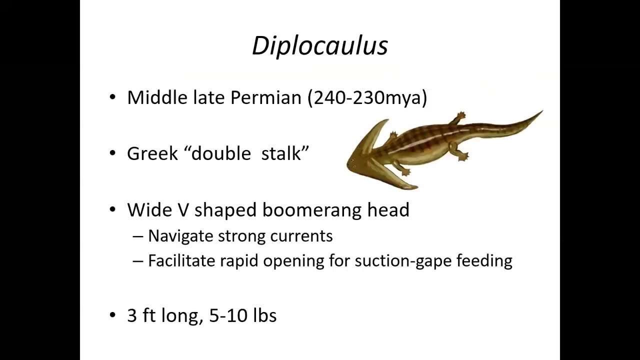 features, but it in fact was an early amphibian. It had both aquatic and terrestrial forms of the Eriops structurally, some features that would appear later in reptiles. So Eriops is a really important fossil, early amphibian fossil from 270 million years ago. And if you think about 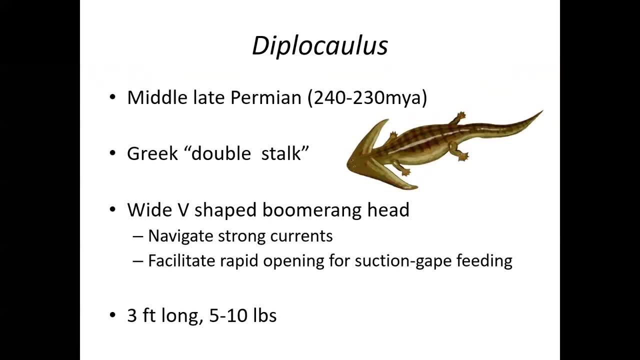 these Lispodondoli. I told you that Diplocallis is perhaps the most famous of all of the Lispodondol early extinct amphibian lineage And obviously the most notable characteristics is a really V-shaped, boomerang-shaped head. This guy was anywhere from three feet long. 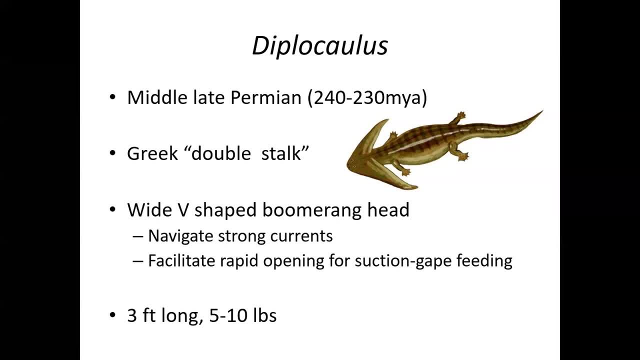 five to ten pounds. It was really one of the largest fossils found in the Lispodondol group, With the thinking is that V-shaped boomerang head helped navigates strong currents and rivers and streams Or, at the same time, agents such as porcelain act as� 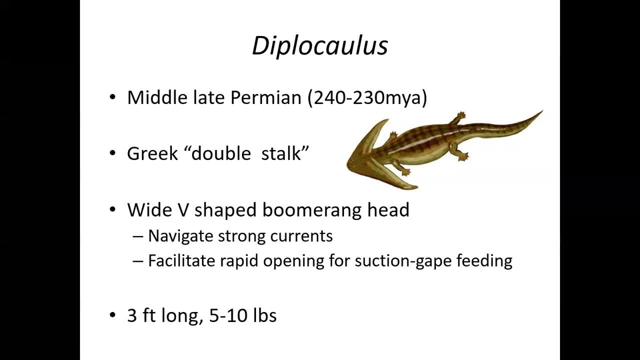 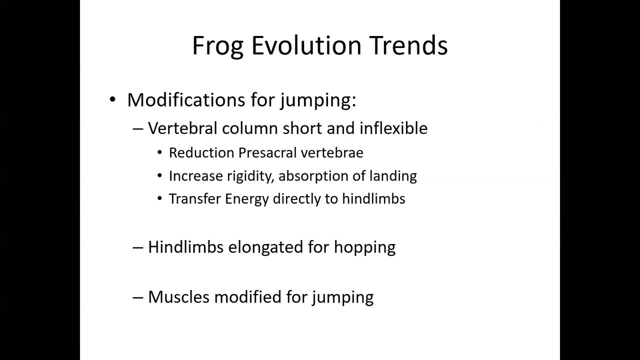 it facilitated the rapid opening for suction gate feeding, which we'll talk about in a couple of lectures. So that's really the main fossils that I want to talk about with regard to amphibian evolution that tend to be more salamander-like. So now let's talk about more of the fossils that 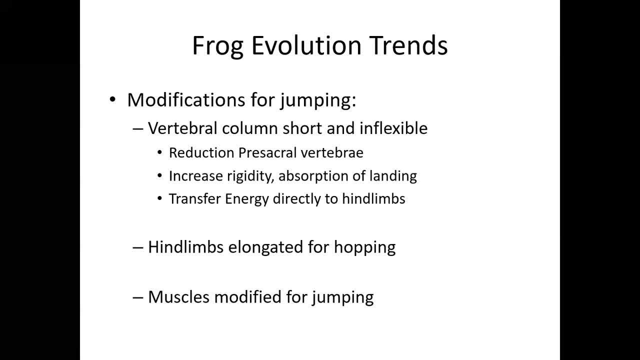 tend to be more anurin or frog and toad-like, And frog and toads have some pretty significant evolutionary developments that differ from salamanders, largely because of the modifications for jumping. If you think about it, they've got vertebral columns that are very short and 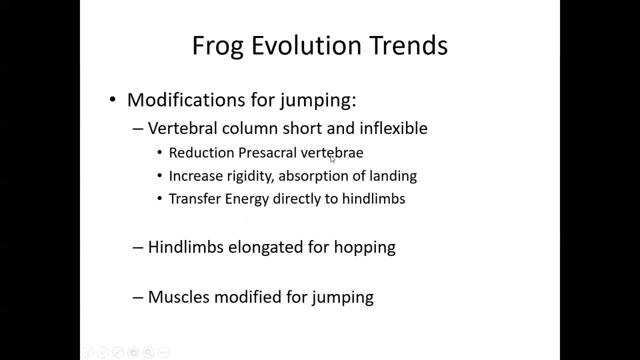 inflexible. So they have a reduction in presacral vertebrae. So those sacral vertebrae are the vertebrae that are found within the pelvis. So here we're talking about a reduction in presacral vertebrae. So those would be the cervical, the thoracic and the lumbar vertebrae. 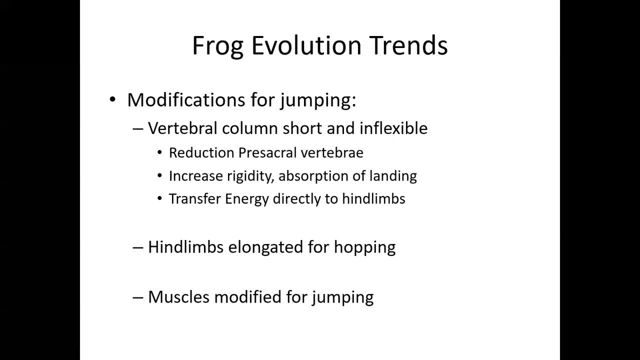 And we tend to see a reduction in those- And Inca decrease rigidity and help absorb the shock when these early frogs were landing, in terms of jumping and transferring of the energy directly to the hind limbs to help with that saltatorial or jumping lifestyle, And, of course, the hind limbs, including the feet, were elongated for 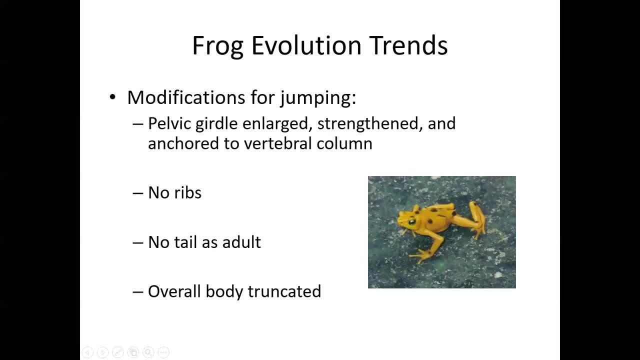 jumping. The muscles were modified for jumping. The pelvic girdle was enlarged, strengthened and anchored to the vertebral column again to help develop that rigidity so that the animals could use most of that energy in their hind legs for jumping. They lack ribs. All but four species of frogs. 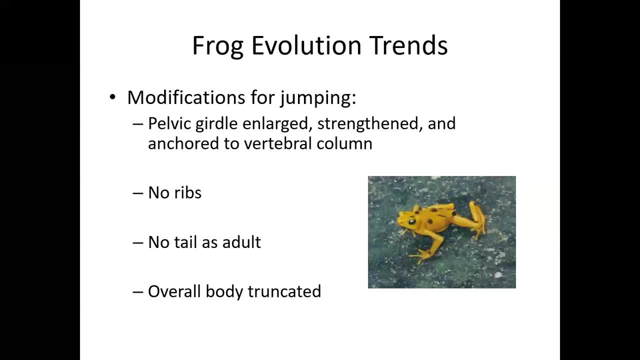 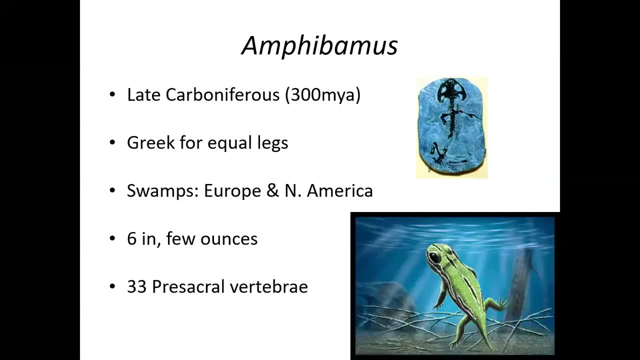 lack tails As adults. there are four species that are up-tailed frog, But overall the body is very truncated relative to that of our salamander counterparts. So let's talk about some of the famous fossils of our very early amphibians that tended to move. 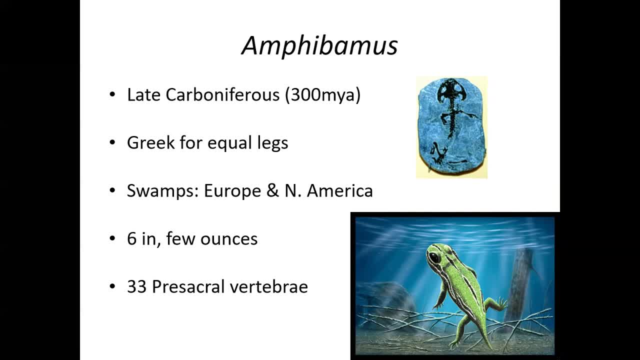 toward our frog lineage. The first of those is Amphibamus. It was found in the Lake Carboniferous. It's a smaller tendospondyline, but it's Greek for equal legs, So the forelimbs are roughly the same length as the hind limbs, which tend to be more salamander-like than frog-like. 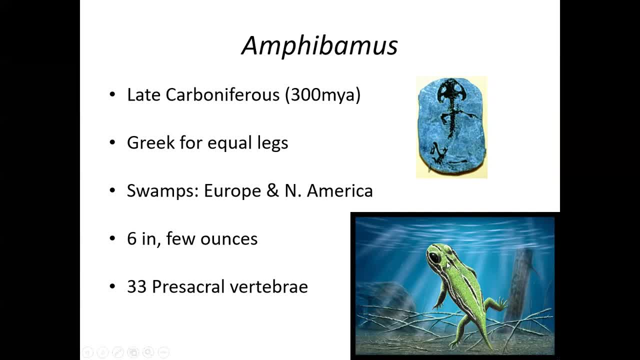 as we're going to continue to learn. It has 33 presacral vertebrae. So, again, this is a really early species that tends to have characteristics, characteristics of amphibians in general, not necessarily just frog, but it does have a wide, frog-shaped head. 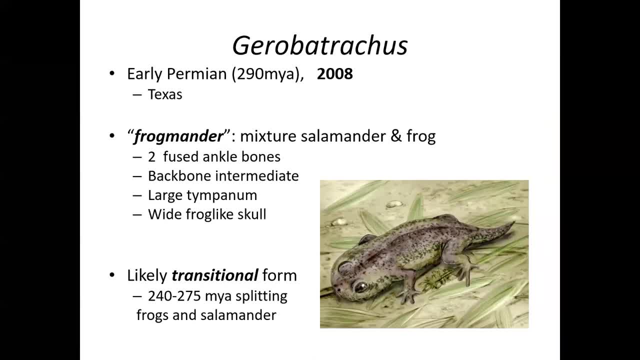 So if we go from 300 million years back, 10 million years earlier or later, in the early Permian we have Gero Batrachus, And this is a mixture. this is our fossil, that's sort of our transitional form between our salamander amphibians and our frog amphibians, And so oftentimes it gets the 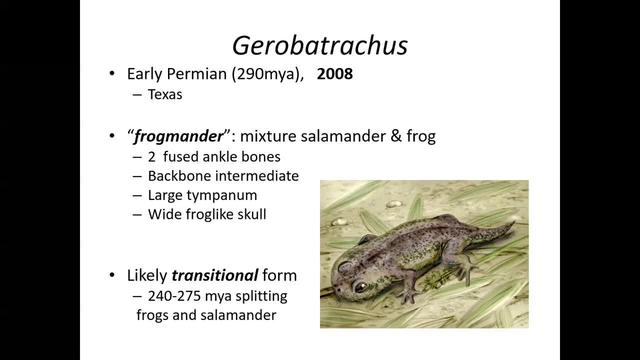 nickname frogmander Because of that mixture of salamander and frog characteristics. So this particular fossil has two fused ankle bones, a backbone that's intermediate in length. So it's a decrease from those 33 vertebrae that we saw on that really early amphibian fossil. 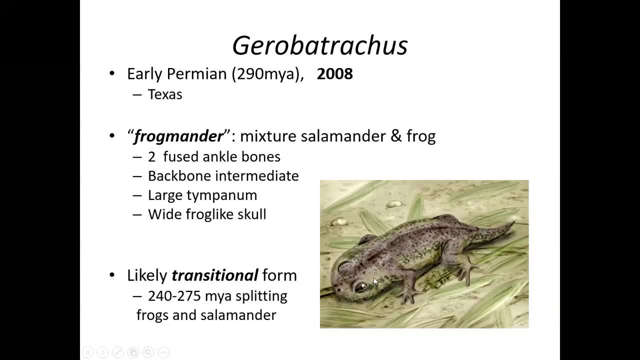 A large tympanum. Remember the tympanum is the external ear on a frog, wide, frog-like scale, wide frog-like skull. Again, this is a transitional form between characteristics that are frog-like and characteristics that are salamander-like. So this is a Gero Batrachus, around 290 million years. 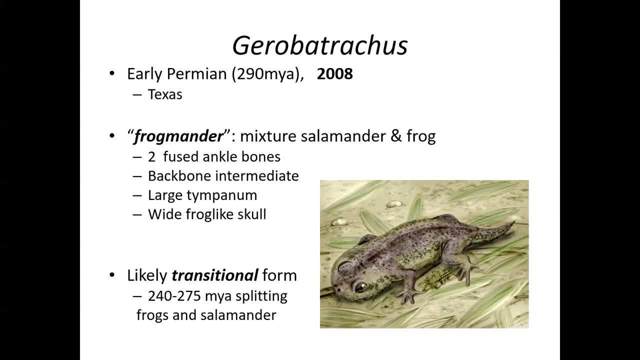 ago. So we think that there's a split between frogs and salamanders anywhere from 240 to 275 million years ago, And that's a really important date that I want you to remember, When the amphibian lineage is split into frogs and salamanders 240,, 275 million years ago, which is predated by this. 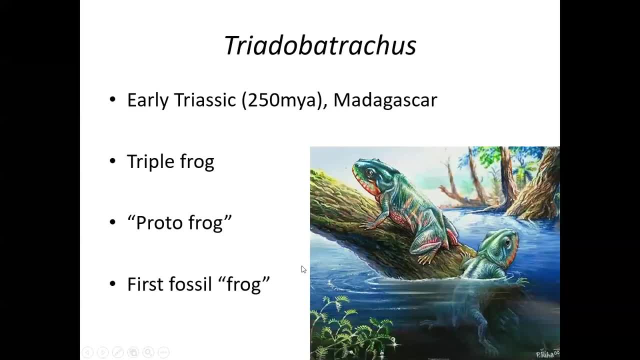 Gero Batrachus, which is that transitional form Now Tridobatrachus, is our first true frog-like fossil, And you can actually see from the artist's rendition that they are tending to start to look a little bit more like our extant. 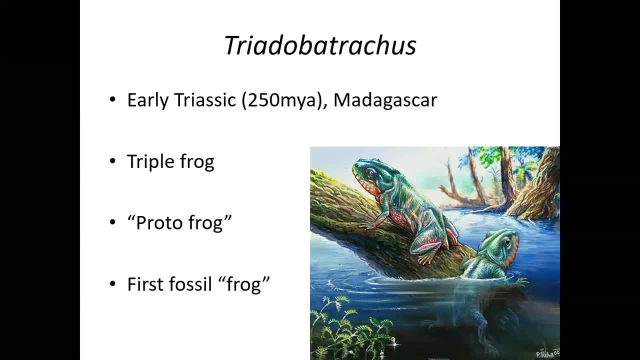 frogs Around 50 million years ago, prior to the next fossil, which is varilla. this particular species or group of animals had short, stubby tails, was clearly a frog. The body size was small, about 10 centimeters in length. The body size was small, about 10 centimeters in length. 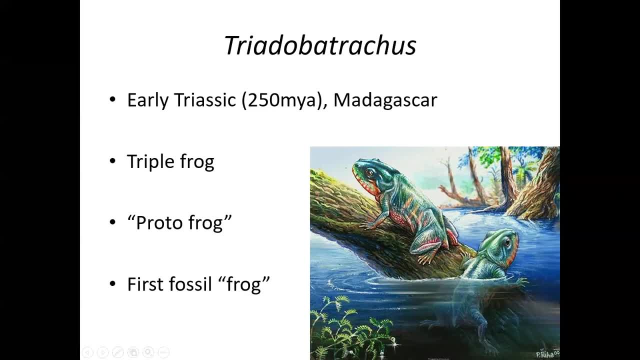 And it differed from modern frogs in that it has 13 or 14 pre-sacral vertebrae compared to nine in modern frogs. So we're going to take a look at the skeleton of Tridobatrachus and compare that to some of the more later more. 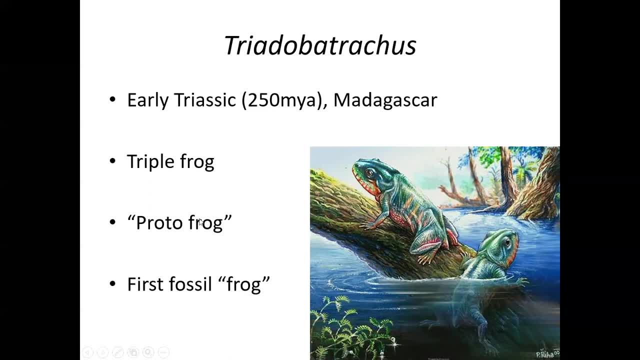 species that resemble more extant frogs. So Tridobatrachus is our proto-frog. It's our first fossil frog where we're starting to see differences between the forelimbs and the hindlimbs, A reduction in the length of the forelimbs and the length of the hindlimbs, A reduction in the 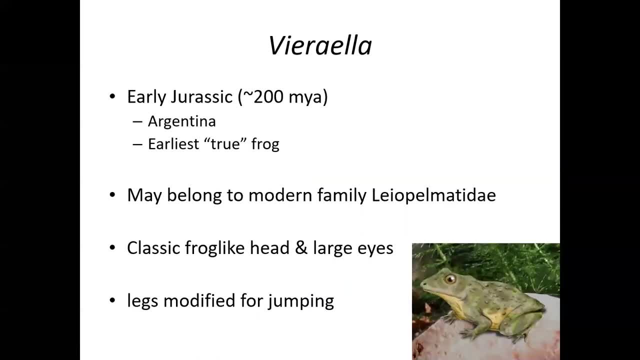 length of the forelimbs and the length of the hindlimbs. We're starting to see differences between the forelimbs and the length of the hindlimbs. We're starting to see differences in the length of the forelimbs and the length of the hindlimbs. Now varilla is found, about 200. 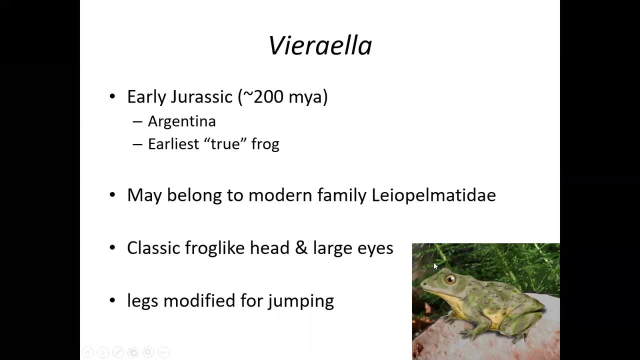 million years ago. It's our earliest true frog And again you can see the artist's rendition. It actually does start to resemble some of our more modern day frogs, particularly the family Lepiochromatidae, which are found in South America, So it's classically a frog-like head. 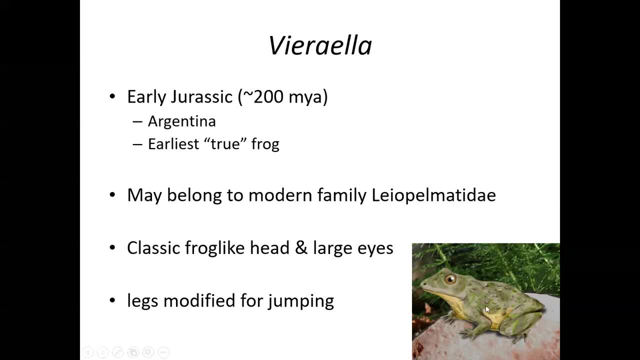 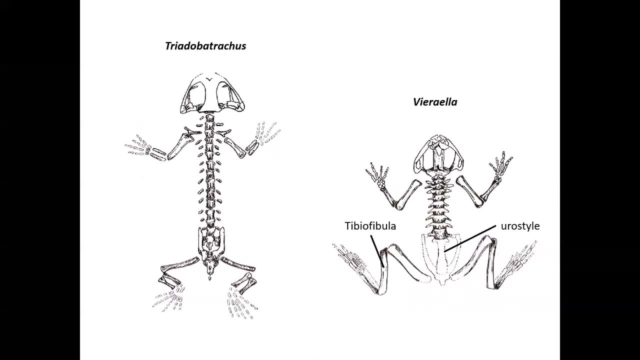 really large eyes, really large, powerful hindlimbs relative to the front limbs, clearly modifications for jumping. So here's that comparison and you will see the same frog. So you will see the schematic again. So there's a couple of things that I want to point out to you. 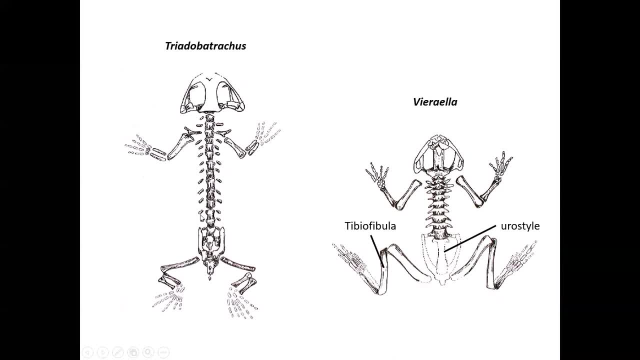 So here's our Trinopatracus, which is that early proto frog, And remember, it should have anywhere from 13 or 14 pre-sacral vertebrae. So it's not the characteristics. The varilla, on the other hand, has nine pre-sacral vertebrae, which is what our current 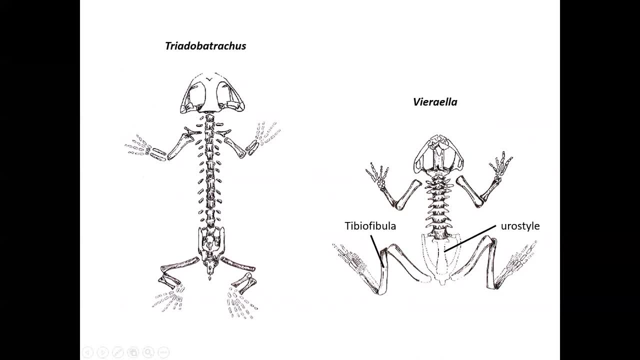 or extant frogs of today have. So that's the first difference. This is reduction in pre-sacral vertebrae in our current frogs, Our proto frog, Trinopatracus, has 13 or 14.. The other thing I 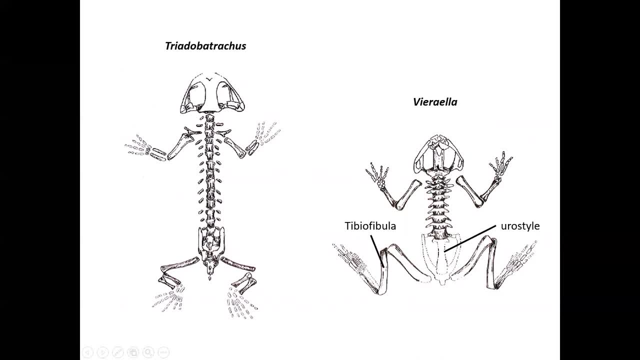 want you to notice is the pelvis itself. And look at the vertebrae, the sacral vertebrae within the pelvis, all still small, relatively ununified, whereas in Virella, very large pelvis and the sacral vertebrae are all fused to form a uro-style. The other thing you should notice if you look at 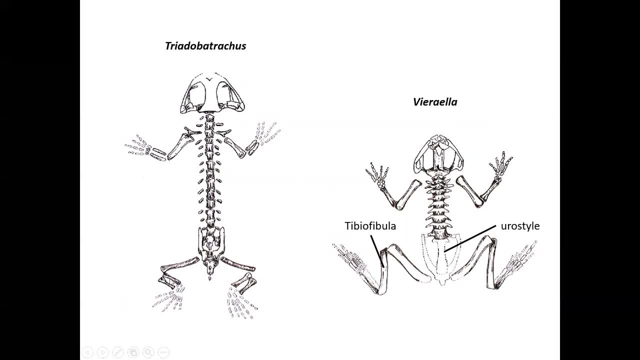 the lower leg bone you have the tibia and the fibula in the Trinopatracus, whereas in the Virella and all extant frogs that we have today have a fused lower leg bones into a tibial fibula Again. 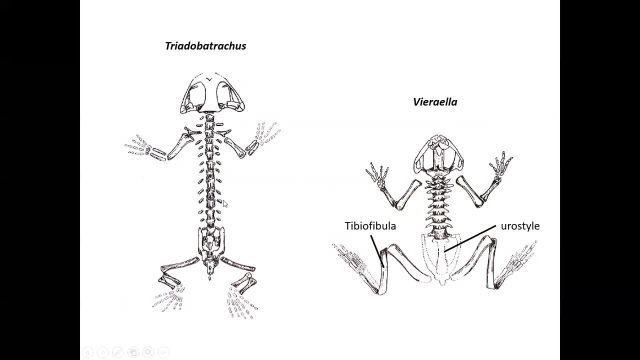 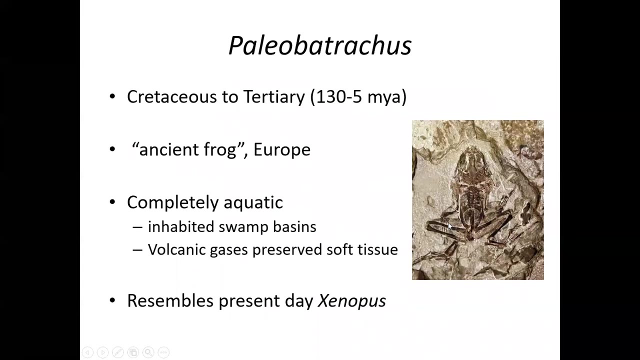 highly adapted for a saltatorial or jumping lifestyle. So, again, I would like for you to be able to point out the various differences between the early proto frog and the very first representation of the extant frog based on the Virella fossil. If we move forward 100 to 135 million years ago, we're looking at Paleomatracus, And this is often 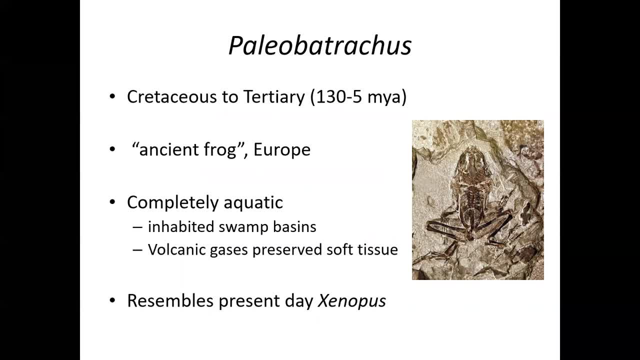 coined as our ancient frog. It was a completely aquatic frog which inhabited our slumps and and other bog areas, And then this particular fossil was preserved by volcanic gases, which actually helped preserve some soft tissue. And this particular fossil, even though it's not directly related, it tends to resemble our present-day Xenopus.